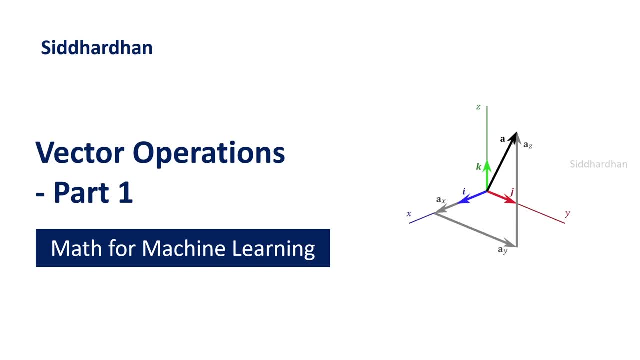 learning course with Python. If you want to learn my course from the beginning, you can go to the playlist section of my youtube channel, so there you will find module wise playlist, So you can start learning my uh course module wise in that playlist. Okay, so, with that being said, let's get. 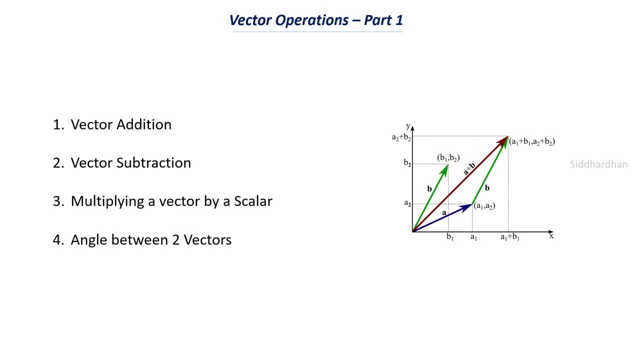 started with today's topics. So these are the topics or the vector operations that we will cover in today's video. So they are about vector addition. so we will see how we can add two vectors with a single vector function. So let's get started with that. 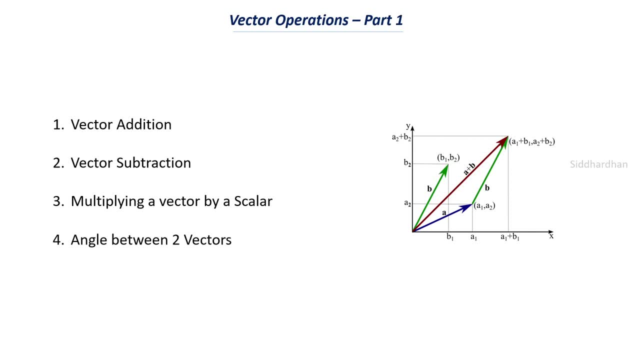 mathematically and also graphically, and how we can do the same for vector separation, and how we can multiply a vector by a scalar. and finally, we will understand what is the significance of an angle between two vectors. So these are the basic operations that we will be seeing in today's 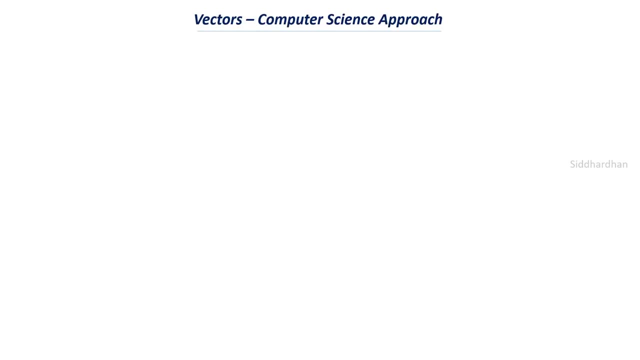 video. okay. So first of all you know, I will just give you a quick recap of what is meant by these vectors when it comes to computer science. So first let's understand about scalar. Scalar is nothing but a number, So it is just an individual number. So it can be 20,, it can be 40 or it can 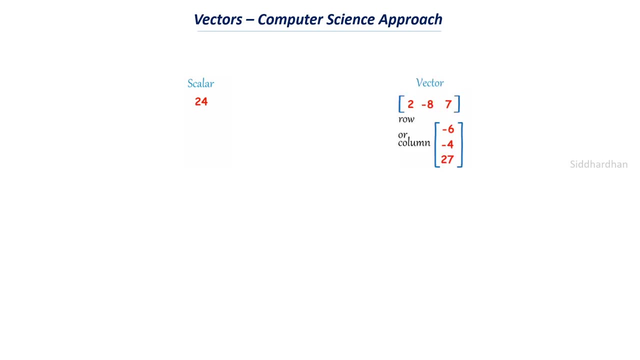 be 100.. It's just only one number, okay, Whereas vectors are nothing but list of numbers. So it can be either a row of- you know- numbers or it can be a column of numbers. So we can have only one row or one column. We cannot have multiple rows and multiple columns. So if we have multiple rows, 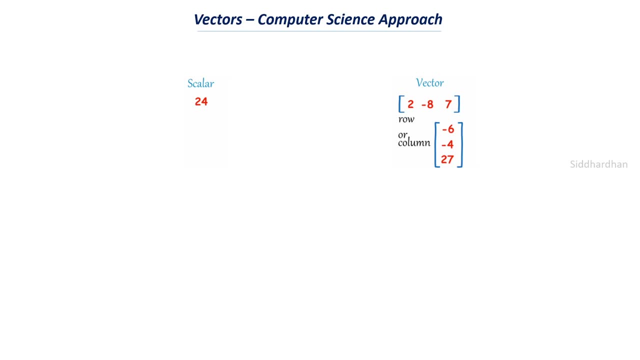 and multiple columns, then it becomes a matrix. When it comes to vector, it contains numbers or values in only one row or in one column. okay, So this is not like you know, our physicist would describe a vector, or a mathematician would describe a vector. So 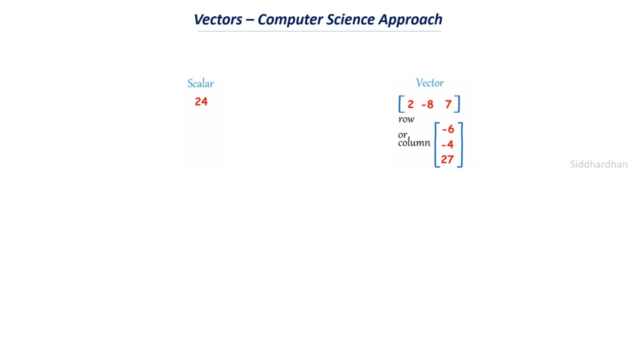 they would say that vector is something that has, you know, both magnitude and direction. But we won't take that definition in computer science. In computer science, vector is something that has multiple numbers. So or you can just consider an array as a vector, okay, So it is very similar to. 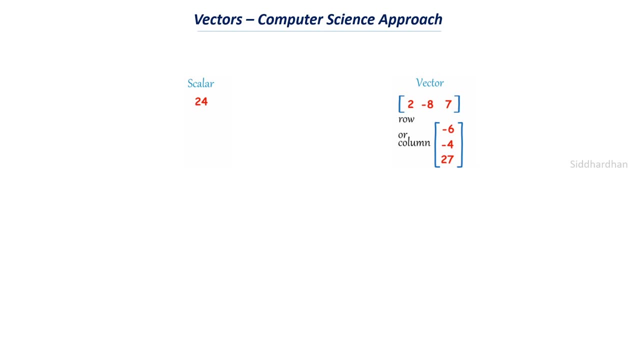 an array in computer science. So now let me explain you what is the significance of vectors in machine learning. Let's say that there is a person and we want to find whether this person has a number or not, and we have this data. So this data represents so the first value here. so you can see. 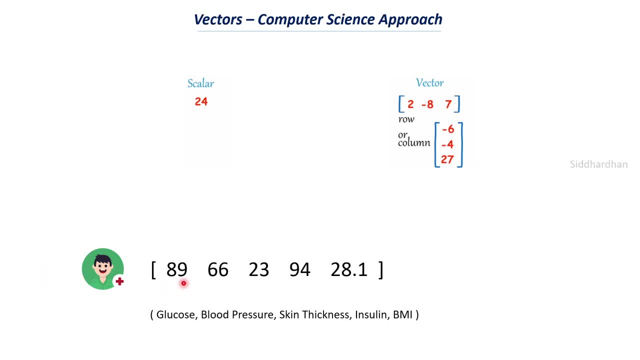 this 89. So just a second So you can see this 89.. So this 89 represents the blood glucose level and 66 represents the blood pressure, 23 is about skin thickness and 94 is insulin and 28.1 is the BMI of. 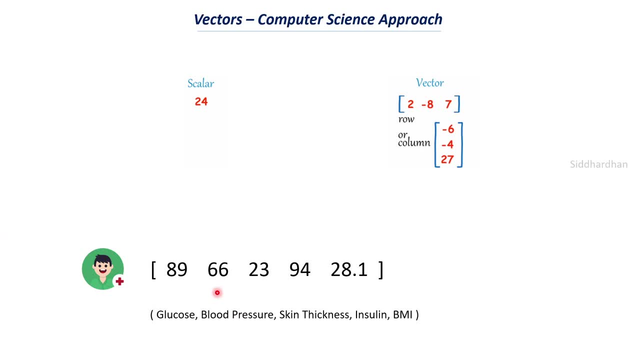 the person. So this is a single data point. So you can see here all these values can be, you know, put in a list, or it can be put in an array. So this particular entity is an example of a vector, because we have understood that vector is nothing, but it is an. 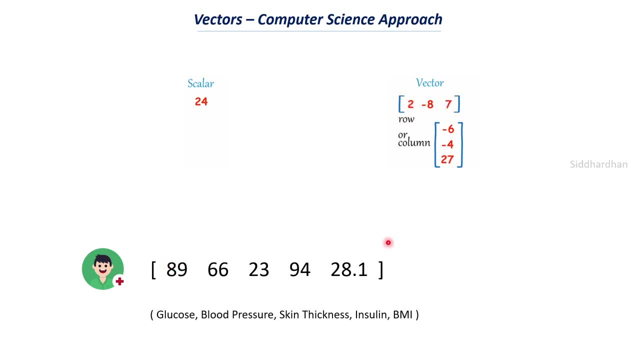 array of values. So you can see here this is also an example of vectors. So this is how data get processed in machine learning. So we will feed this data set to a machine learning model. So the difference is that we will use several data points, but each of this data point or each of this, 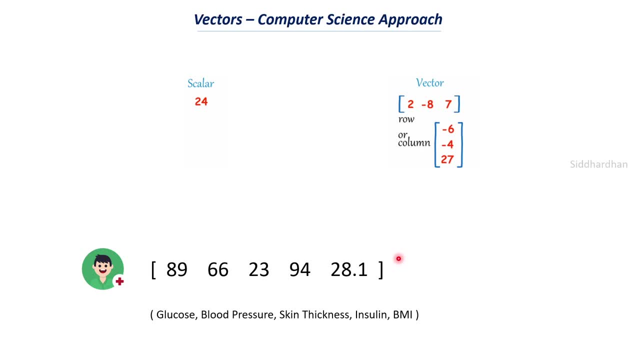 you know, row or entity is an example of a vector. Hence it is very important to you know, know about all the different operations that occurs in a vector to understand how the computation works. So all the computation that goes inside a machine learning model will be based on these vectors. So 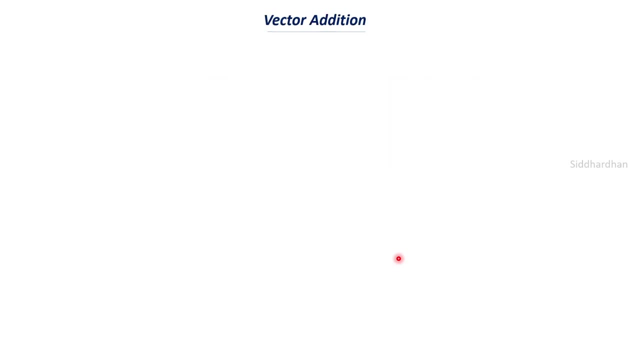 understanding. this is very important. So now let's understand vector addition. Let's say that there are two axes, So one is the x1 axis and x2 axis. So in machine learning we, you know, sometimes the variable y is used for the target variable. So in the previous case you can see here that we wanted 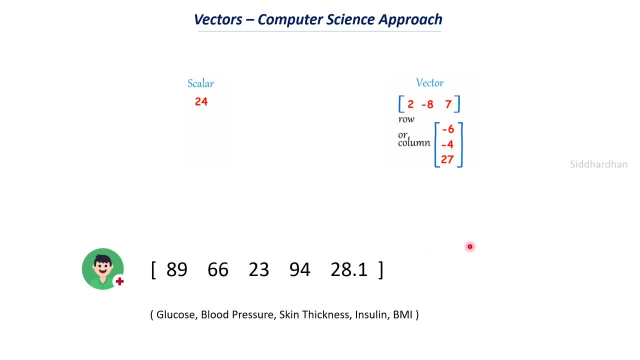 to predict whether the person has diabetes or not, right? So that prediction, whether it is yes or no, the y variable. So this is the target variable. So we won't take the y axis here. So instead of that, we will take the axis as x1 and x2 instead of x axis and y axis. Okay, so that's the reason. 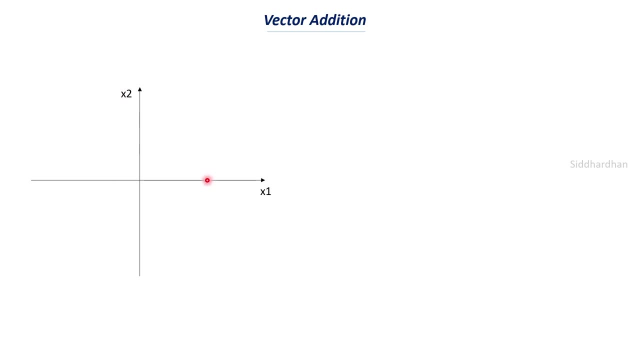 So it is not that significant. So in this x1 and x2 coordinate we have a vector, and this vector is 2 comma 3.. So this is nothing but this point. So you can see this arrow here and if you take this point, it is the coordinate of this point is nothing but the vector, So 2 comma 3.. So it means. 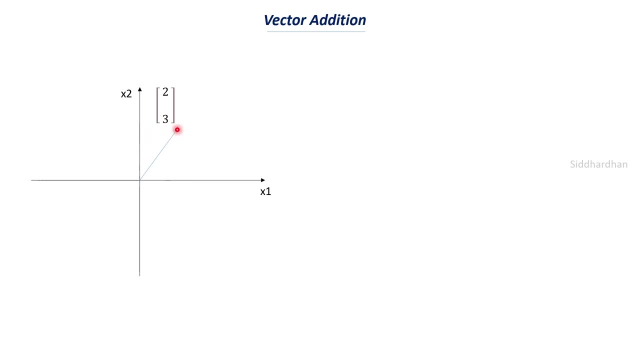 that there is two units in this x axis and three units in this x axis. So this is the x axis and three units in this y axis. So it is this point. So this is an example of a vector. So there is another vector, So this is nothing but three units in this x axis in the positive x direction, minus. 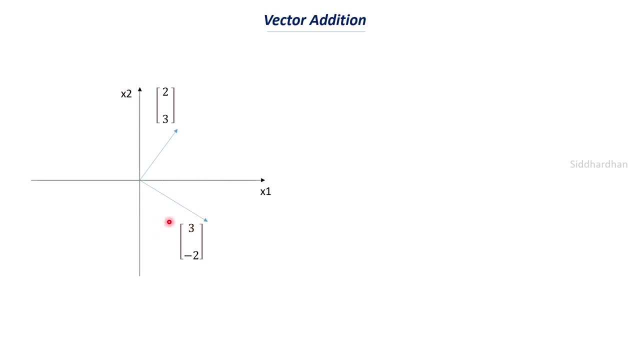 2 in negative y direction or negative x2 direction. So here there is a point, and the coordinates of this point is nothing but 3 comma minus 2.. So now we have two vectors. Okay, and now we need to add two vectors: This 2 comma 3 vector and the 3 comma minus 2 vector. Okay, so now let's see what is the. 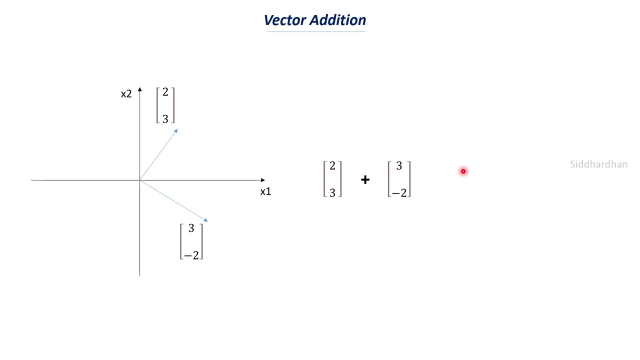 result we can get if we, you know, add two vectors. So now let us see what is the result. we can get two vectors and the important point to note here is the vector should be, you know, in a same shape to add two values. Let's say that we have three values in one vector. So two, three and one. let's. 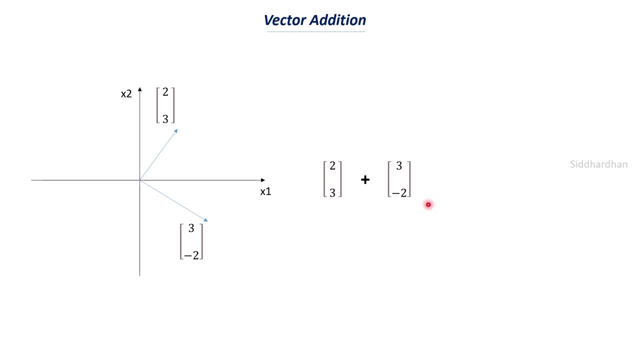 say that we have three values in this vector and two values in this vector, So we cannot add vectors which are, you know, which don't have a same shape. So in this case the two vectors have same shape, So both of them have two values. So like that we can add vectors only if the number 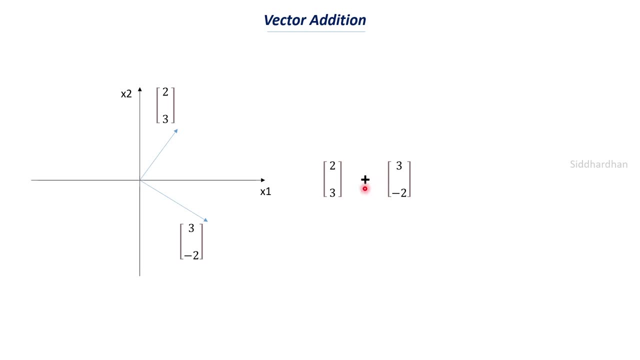 of elements is the same in both the vectors. Okay, so now what we are going to do is we are going to do is we will do element wise addition. So this 2 will be added to this 3 and this 3 will be added. 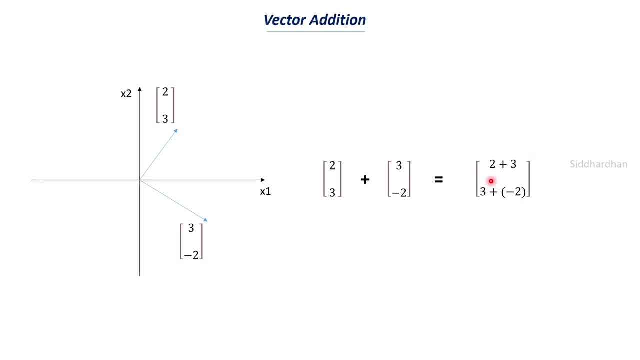 to minus 2.. So you can see, here it is just elemental addition, simple elemental addition, and when we add it we will get this 5 comma 1 or 5: 1, as are the result of this addition of two vectors. Okay, so this is the resultant vector. Now, instead of doing this, you can also get this: 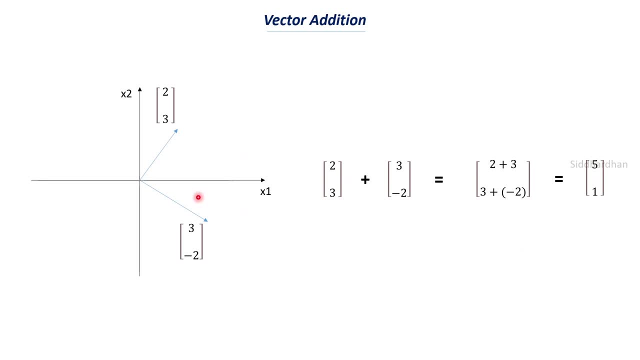 result and the addition of these two vectors from this graph. So what we can do here is you can draw this daughter lines, So you can take this point- So this is second vector point- and just draw a daughter line and from here also you can draw a daughter line. So now we can. 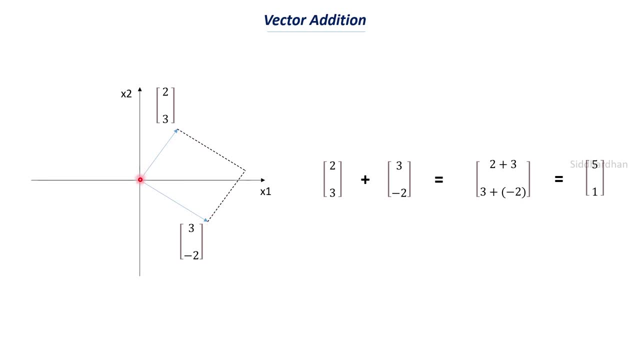 get this rectangle and then you can join this diagonal. So this point and this point, So this will be our addition of two vectors. So if we, if you take these two vectors and if you- just, you know- join through daughter lines, and if you take the diagonal and this diagonal becomes a 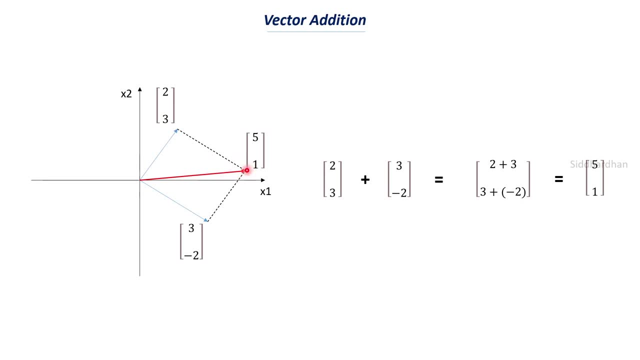 the resultant addition of the two vectors. So you can see here, if you take this point and the value of this point will be 5, 1 to 1.. So this is how you can add two vectors and you can, you know, do this either mathematically or instead of that, you. 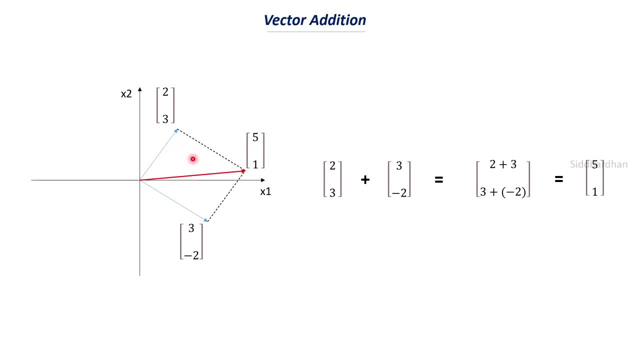 can also find it graphically in plotting in a graph. Okay, so this is how we can add two vectors. So the main thing to note here is: in vector addition, the values will be added element twice and the shape of the vector should be equal for both the vectors. Then only we can. 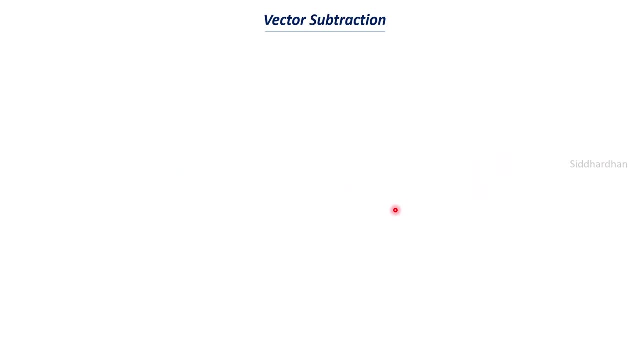 do addition. Okay, so now let us discuss about vector subtraction. So I will just take the same vector, which is 2 comma 3 and 3 comma minus 2.. So we have this x1 axis and x2 axis and we have the 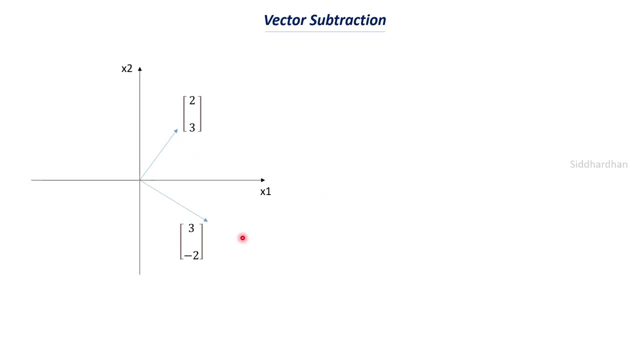 first vector, which is 2 comma 3, and the second vector is 3 comma minus 2.. So it is very similar to vector addition and here also so when we do this subtraction. so both of the vectors should have the same shape and here also it is element twice subtraction. Okay, so here it will, this: 2. 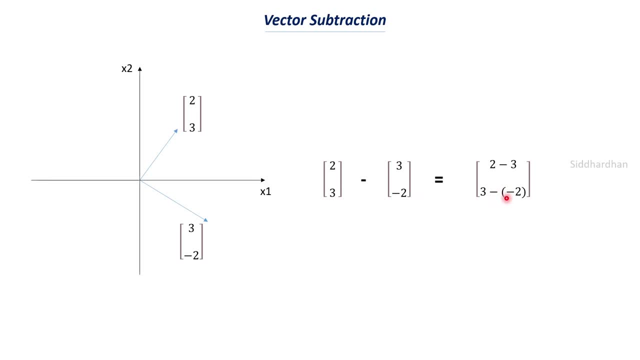 minus 3 will be the resultant of this first value, and 3 minus minus 2, you can see a minus of minus 2, and the resultant which we will get is 2 comma 5.. So this is our resultant vector. So, and there is another thing, if you add two vectors, 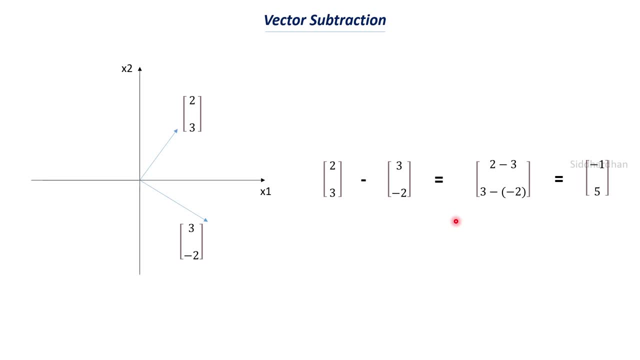 you will get a vector, you do not get a scalar, Okay. and also, if you subtract two vectors, the resultant will be a vector and it will not be a scalar. Okay, so these are very basic things, but we may, you know, kind of forget about this, but they are these small things which we need to you. 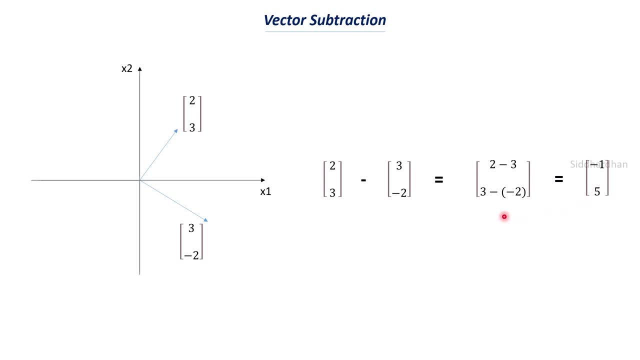 know, remember. So when you add two vectors, we will get a vector, and also it is the same for subtraction. Okay, so the resultant which we are getting is minus 5.. So now let me explain you how can do this graphically. Okay, so you can see, here we are subtracting the second vector from the first. 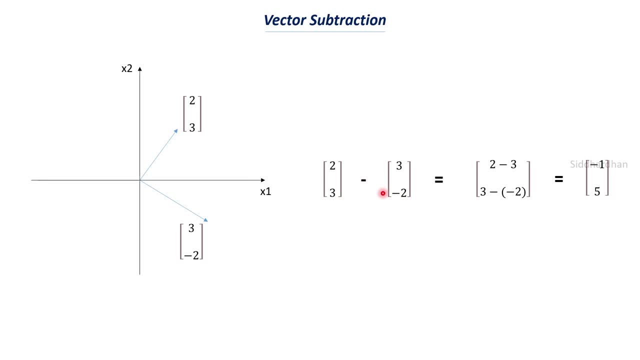 vector right. So when you have this minus sign, you need to reverse this vector. So you know, when you reverse this vector, what you will get is minus 3 and plus 2.. So the reverse vector will be this. So it should be the same magnitude, but exactly in the opposite direction, just 180 degree. 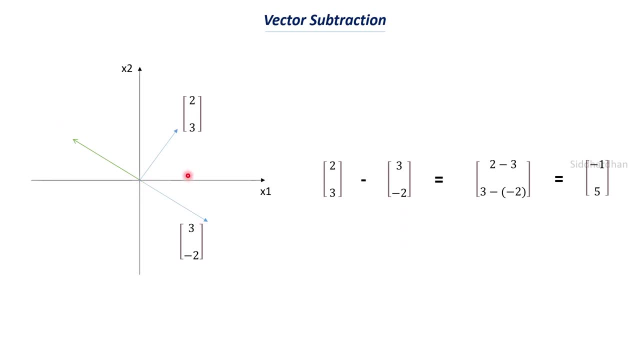 So it is the exact same vector, but in the opposite direction. Now, what you can do is you can again, you know, join these dotted lines, as we have did before. This is the normal vector vector and this is the diagonal vector. so this diagonal will give you 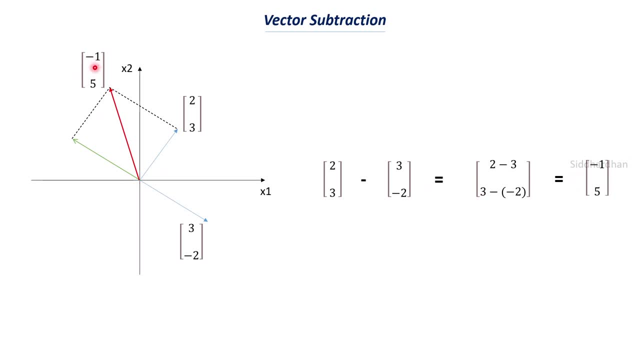 the difference between the two vectors. You know the subtracted value of these two vectors. so the value which we got mathematically is minus 1 comma 5, and when you plot this you will also get this value, which is this diagonal, and that value is minus 1 comma 5.. So this is how you can subtract. 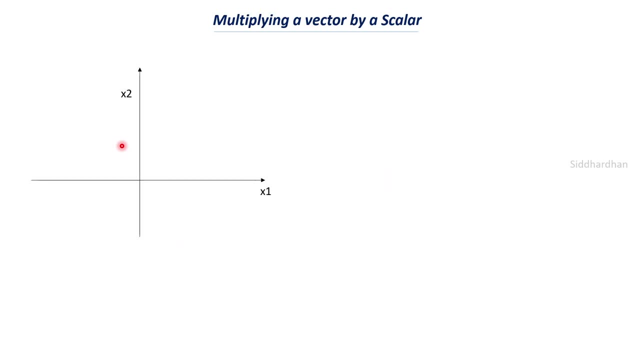 two vectors. Okay. so the next thing which we are going to discuss is multiplying a vector by a scalar. So again, we are taking this x1 axis and x2 axis and we have this vector 2 comma 3. now let's see what happens when we multiply the vector and get this x1, x2, x2, and then there is this vector here, the vector here. 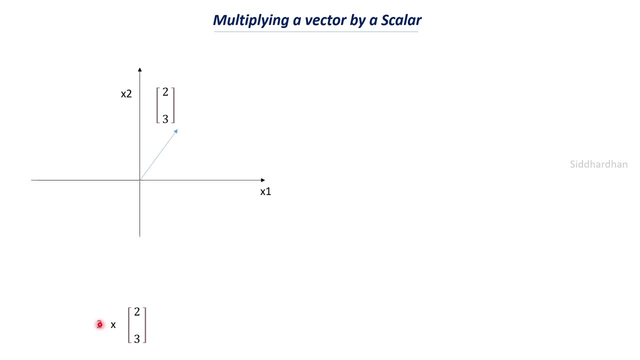 a scalar. so scale. we know that scalar is nothing but an individual number. so when we multiply this individual number with a vector, so the resultant will also be a vector. but what is the difference here is, when you multiply a vector by a scalar, your vector can can get enlarged, or it can get. 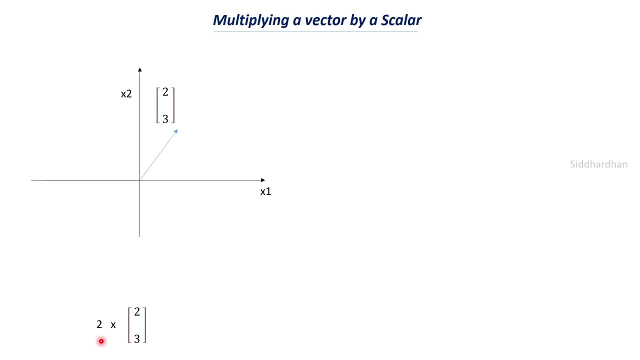 shrunk. okay, so we either enlarge a vector or we shrink a vector. so it is all about scaling. so i'll just explain you this graphically. so when you just multiply an integer or a- you know- a numerical value with this vector, so this value will be multiplied with all the elements of this. 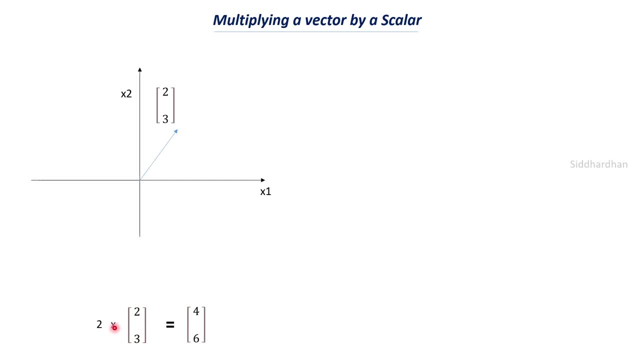 vector. so the resultant which we will get is 4 comma 6, because like 2 into 2 is 4, and this 2 into this 3 will be 6, so all the elements of this vector will be multiplied by this scalar. so this: 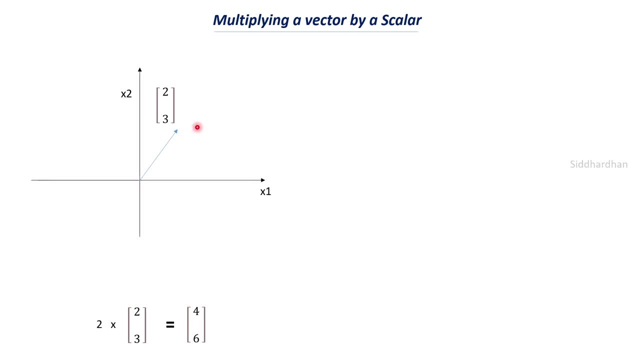 resultant is 4 comma 6. so when you plot this 4 comma 6 in your graph, you will get this. so this vector is enlarged, so it is double the size of the initial vector. and the main thing to note here is the vector which we got will be in. 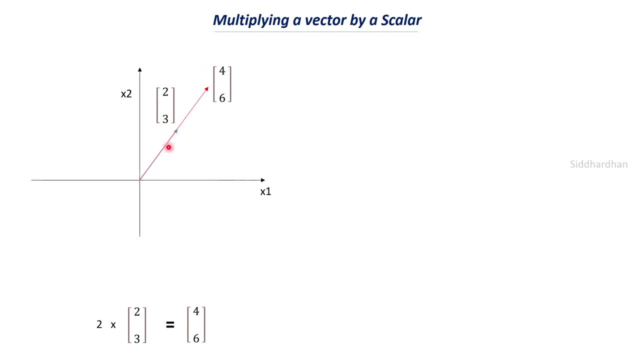 the same direction as that of the previous vector. okay, because, like the values are similar, it is just enlarged. okay, so it will be in the same direction as that of the original vector. so in case, let's say that you have multiplied it with 0.5, so in that case your value will be 1 and 1.5. 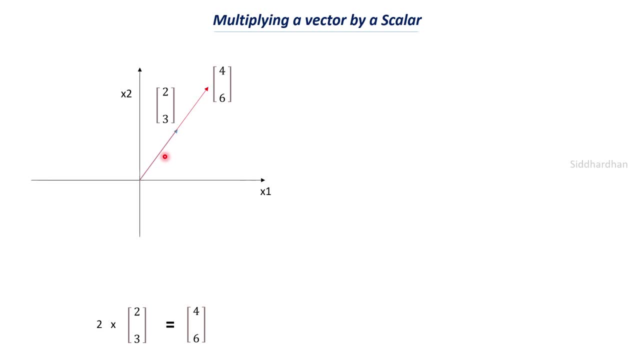 right. so in that case, so you will get a vector here. okay, so your vector will be, you know, reduced in size by half. okay, so when you multiply it by 0.5. now let's take another example. so there is a vector, this 2 comma 3, and now we are multiplying it with minus 0.5. so in this case, what happens is: 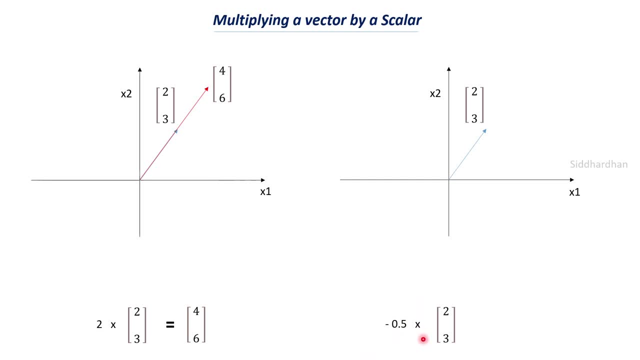 as i have told you earlier, when there is minus sign we need to reverse the vector. so you know, when you just do it mathematically, the value which you will get is minus 1 and minus 1.5. so minus 0.5 into 2 is minus 1, and minus 0.5 into 3 is minus 1.5, right? so when you just plot this in, 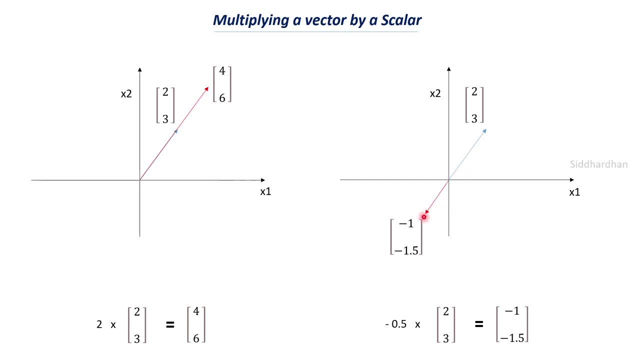 your graph. so this is the point which you will get. so this is the point which you will get. so this is the way which you will get. so here you can see. here it is in the same line, but the direction is reversed because we have this, a negative sign- here, so that the negative sign will reverse your vector. 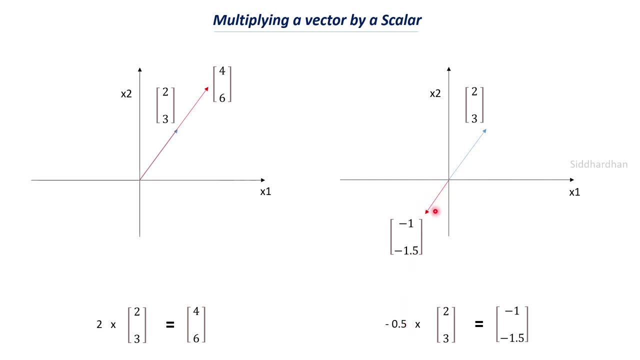 okay, and as we have this 0.5, the size of the vector will be reduced. so this is how you can multiply a vector by a scalar, and there is- so this is also another thing- uh, that, uh, when you multiply a vector by a scalar, you will, the resultant will also be a vector. okay, so it won't be a scalar. 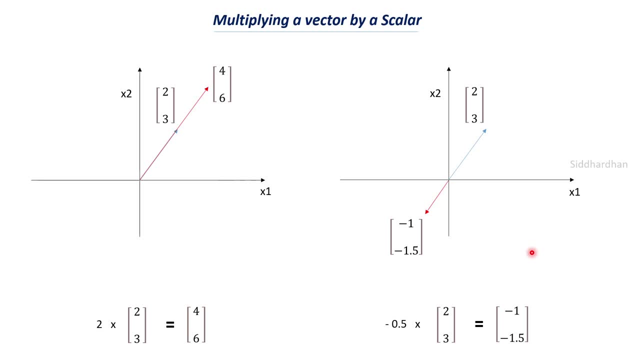 value, it will be a vector value, okay, so this is how you can consider. you can multiply a vector by a scalar. and finally, let us understand what is the significance of angle between two vectors. so we have this again, have this x1 axis and x2 axis, and here we have. 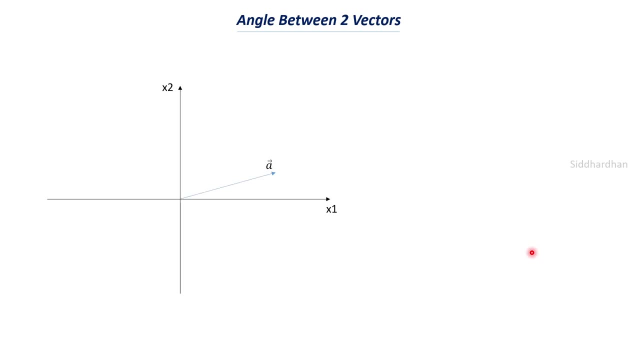 a vector, so this is nothing but a vector. so let us name this vector as a vector. and there is another b vector and also x vector. so the significant point here is the angle between this a vector and b vector. so let it be theta, and the angle between this x vector and a vector. let 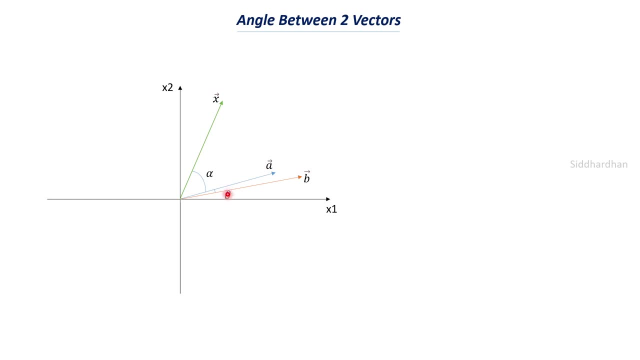 it be alpha. so here you can see. here this angle, this theta angle is very less than alpha. so when the angle between two vectors is very, very small, then these two vectors are very similar to each other, whereas in this case the angle between the c a vector and x vector is very large. so in that, 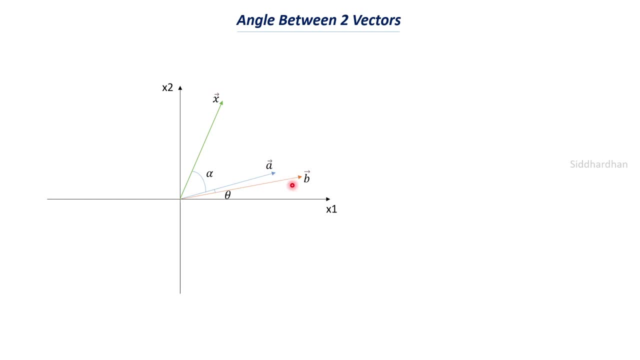 case, these two vectors will be very different, whereas the c a vector and b vector will be very similar. so what is the significance of this? is so, when you have a, when you have two data points- so previously we have discussed about a person having diabetes, right? so when there are two? 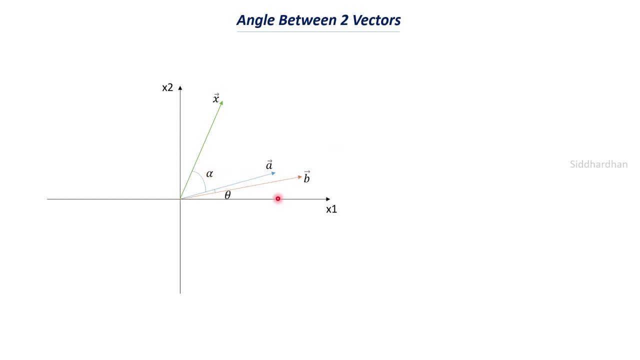 persons and if you plot those values in uh in in graph and if you find that if the angle between those two- uh, you know data points are like the angle between those two vectors, are very small, that means both of the person have similar kind of values, so similar kind of, you know, health values.